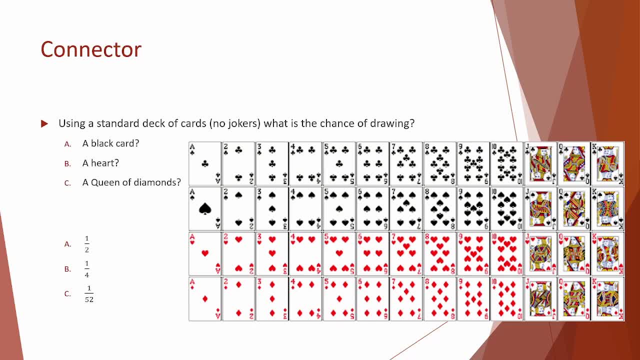 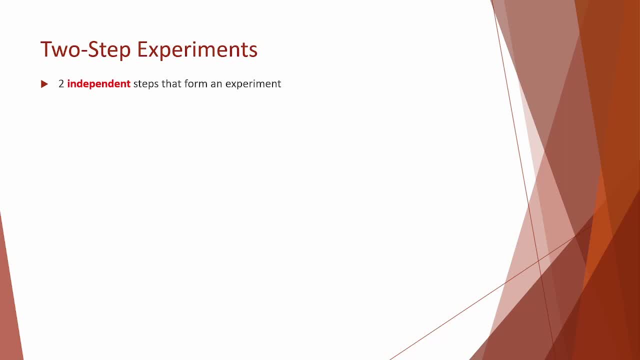 one queen of diamonds out of all of the 52 cards in a deck of cards. Two-step experiments are when there are two independent probability experiments happening that form the total experiment. So each of the steps do not directly affect each other. We can use a table to represent the sample space. 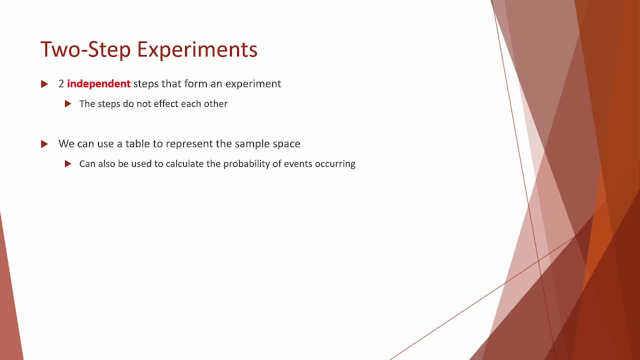 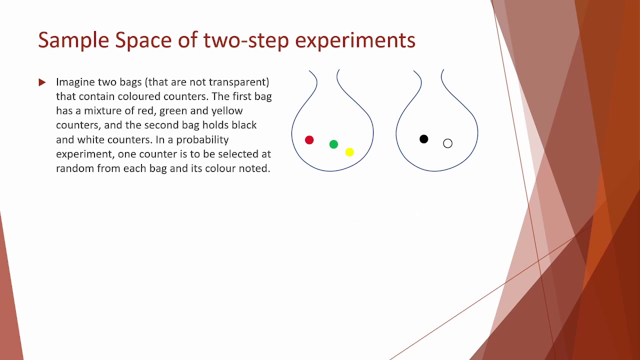 and we can then use that table to calculate the probability of those events happening. So some examples of two-step experiments are whipping a coin and rolling the dice, picking a token from different bags or rolling two independent dice. So here's an example. We have two bags. One bag has a red, a green and a yellow token in it, and one bag has a. 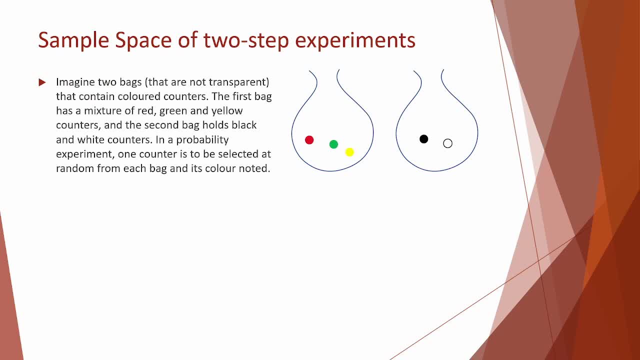 white and a black token in it. Now we can't see in these bags and when we draw out the tokens we cannot tell the difference between the two. So we can't see the difference between the two. So we can't see the difference between the tokens until they're drawn out. So we can create a sample space. 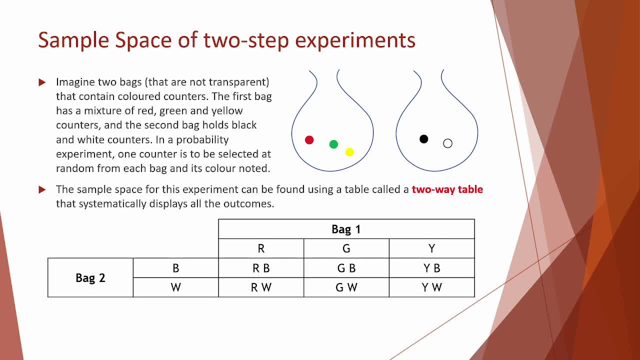 using a table. So for bag one, I've got my red, green and yellow. For bag two, I've got my black and white. I can represent it in the table that is on the screen. I've got red, black as one option. 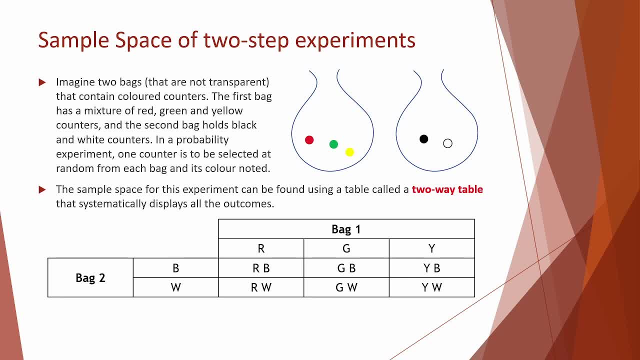 I've got green black as another option and I've got yellow black as the third option, And I could also pick out a red and a white, a green and a white and a yellow and a white. I can also pick out a red and a white, a green and a white and a yellow and a white. 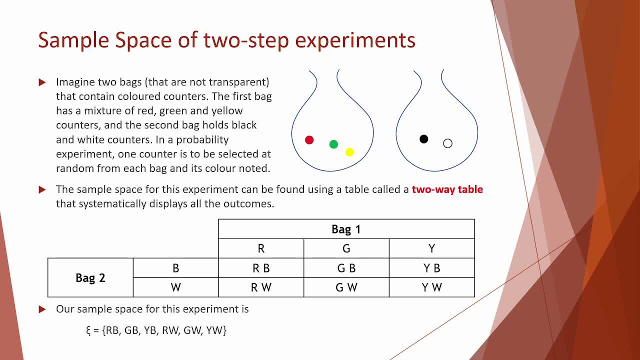 So I can write out the sample space for this by using the set notation. So I've got my sample space. character there equals curly brackets to say: this is the set of and I've got all six of those options in my sample space. Let's have a look at a couple of questions that you might get. 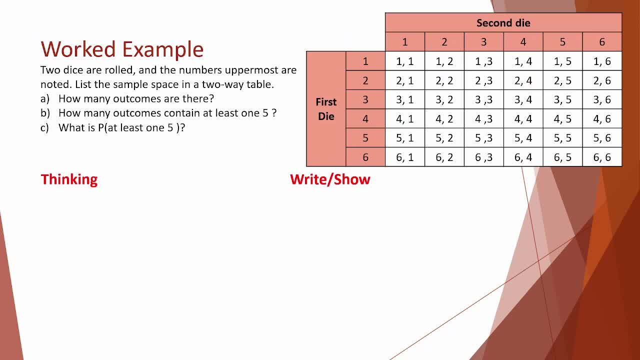 So I've got this example here where I've rolled two dice and when I've rolled the dice I've recorded the numbers on each of the dice. So down the left hand side I've got the first dice, across the top I've got my second dice. and these are all the options, So I could get a one and a one. 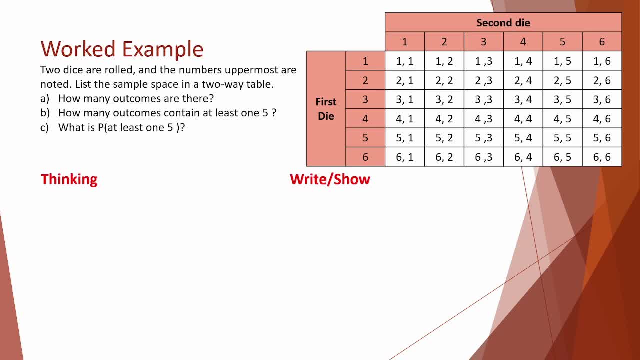 or a one and a two, and so on All the way through to six and a six. So here have my questions. I've been asked how many outcomes there are, how many outcomes contain at least one five, and what is the probability of getting at least 15.. On the left, I've got my thinking and on my right I've got what.